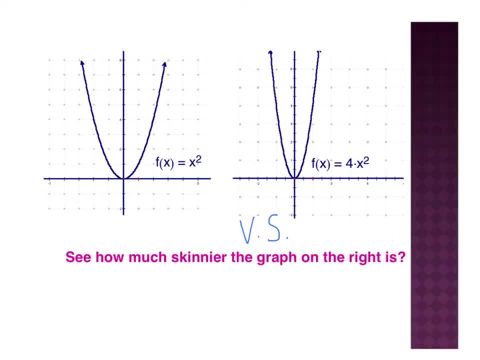 So I have a vertical stretch and usually we notate that with a vs. So vertical stretch. Now this 4 is also important. What I'm doing is a vertical stretch by a factor of 4.. So vertical stretch by 4, meaning my graph is being stretched vertically by a factor of 4.. Now let's take a look at what a compression would look like This time. out in front, I have a 1 third in front of the x squared. Once again, this 1 third is not being affected by my squared part out there. 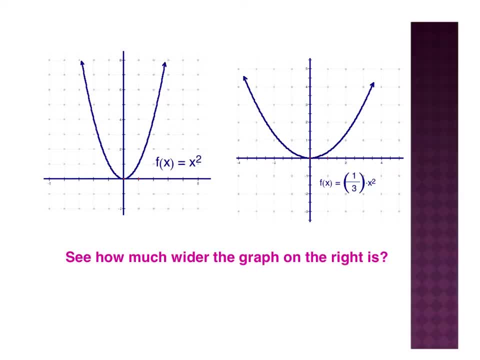 That 1 third is not being squared. Okay, even though the 1 third is in parentheses, it's not in the parentheses that are being affected by the squared. That's very, very important. So this 1 third is not being squared. I can't say that enough. Well, that 1 third being out in front, I know that it's a vertical and because it's 1 third, it's between 0 and 1, it's a compression. So when I'm between 0 and 1, I have a compression. When I'm greater than 1, it's a stretch when I'm talking about my factor. So I have a vertical compression. 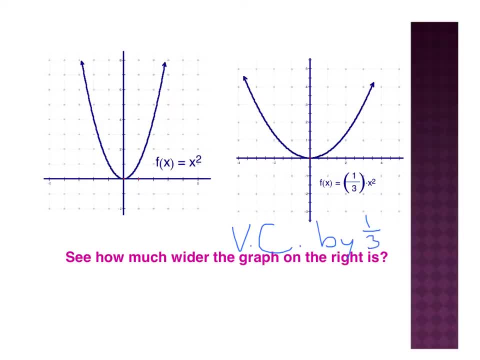 By a factor of 1 third. And again it's a vertical compression by a factor of 1 third. That's very important because when we talk about horizontal stretching compression, you have to think opposite. So it's not necessarily the number that you see, it's the factor that we're using. So here we have a vertical compression by a factor of 1 third. Notice how it gets a bit wider. It's being smushed down, so it's like I have a weight on top of it. that's smushing this graph down. Quick rule to remember: 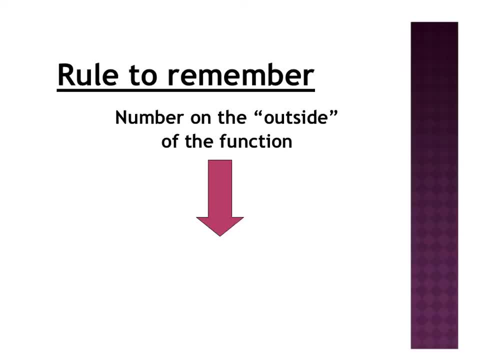 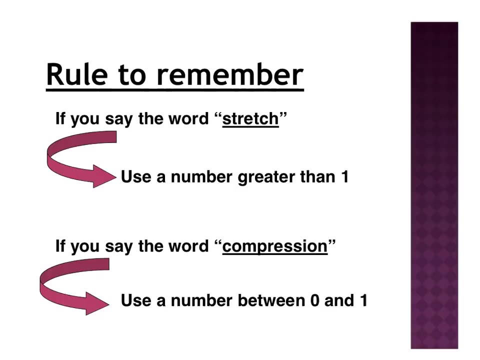 If the number is outside the function, meaning it's outside the part that's being squared, It's outside the square root, It's outside my absolute value, because we'll see all different types of functions. We know that it is a vertical transformation. Another important rule to remember when we're dealing with compression and stretch: If we are saying the word stretch right here, we need to make sure that we're using a number that's greater than 1.. 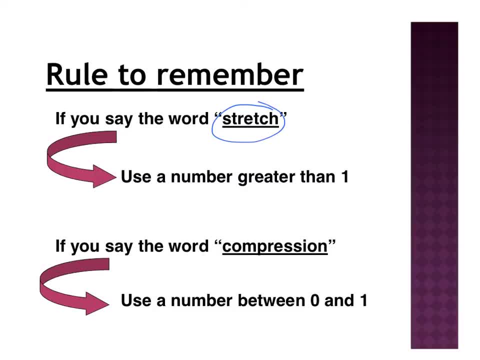 So we'd say a vertical stretch by a factor of 1 third. We wouldn't say a vertical stretch by a factor of 3 or by a factor of 2.. We wouldn't say a vertical stretch by a factor of 1 half. That wouldn't make sense. 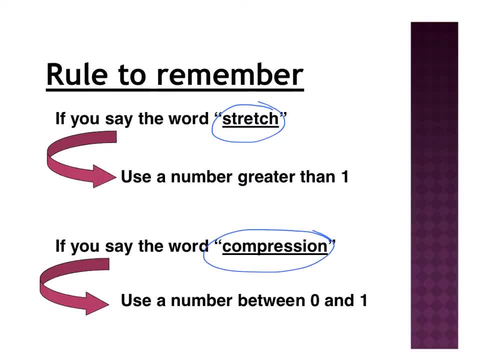 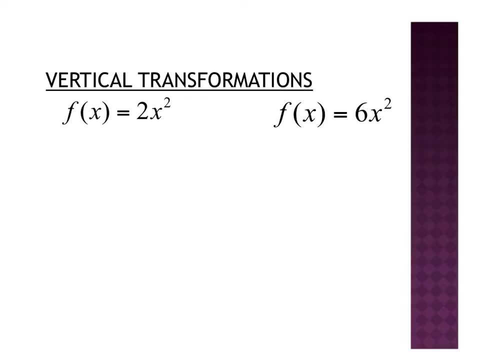 If it's a compression, if we're saying a vertical compression, it'd be a number between 0 and 1.. So we could say a vertical compression by a factor of 1 half or by a factor of 1 third. Now let's take a look at a couple examples for vertical transformations. If we're looking at this first one, here we have a 2 out in front of the x squared. Now that 2 is not being squared, remember, it's just out in front of the x squared. 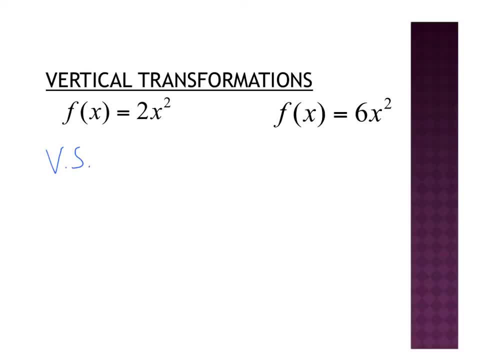 Therefore we have a vertical stretch by a factor of 2.. Let's take a look at this next one. Once again, we have a coefficient out in front of the x squared, So the 6 is not being squared, So I have a vertical stretch by a factor of 6.. 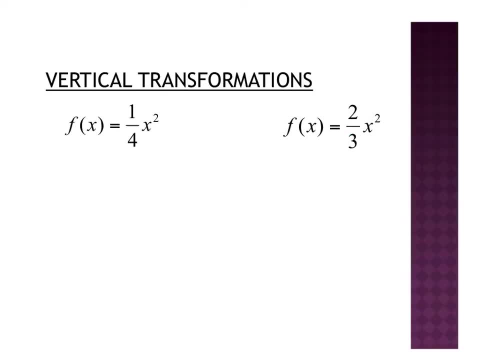 Here we have a couple more vertical transformations. Out in front of this one we have a 1 fourth. So this is still vertical because it's not the part that's being squared, That 1 fourth is not being squared. So I have a vertical and since I'm going to be using 1 fourth, I'm going to say a vertical compression by a factor of 1 fourth. 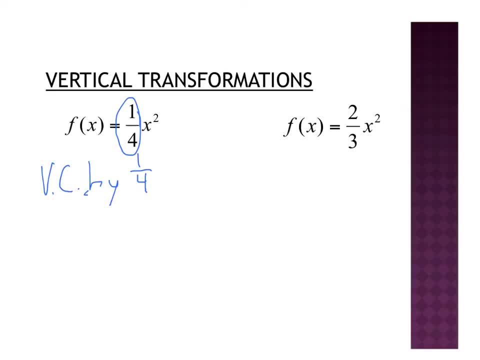 Remember, when it's between 0 and 1, it's a vertical compression or horizontal compression. When it's between 0 and 1, it's a compression. When it's greater than 1, it's a stretch. So let's look at this one. We have 2 thirds. 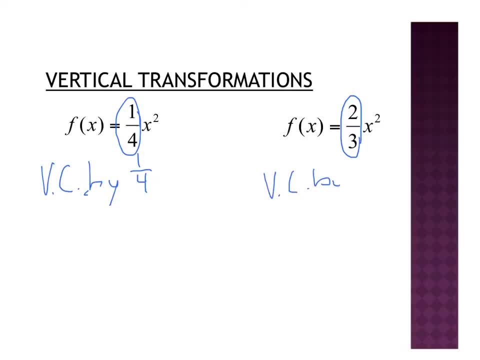 Well, this is going to be a vertical compression by 2 thirds, By a factor of 2 thirds. Alright, now we have a couple combos. Now that's fun. So this first one: we have a coefficient out in front of the x squared. 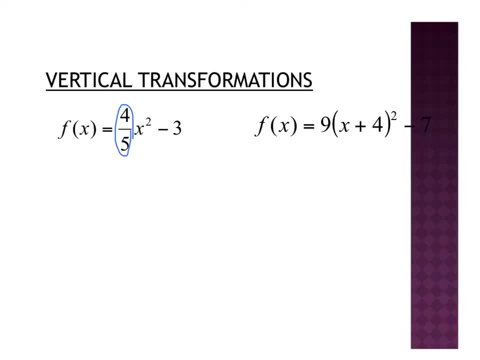 Remember, when it's multiplication, we're talking about stretch or compression. Well, 4 fifths is between 0 and 1, so I have a vertical compression by a factor of 4 fifths. Over here I've got a minus 3.. Now that minus 3 is outside the squared part. 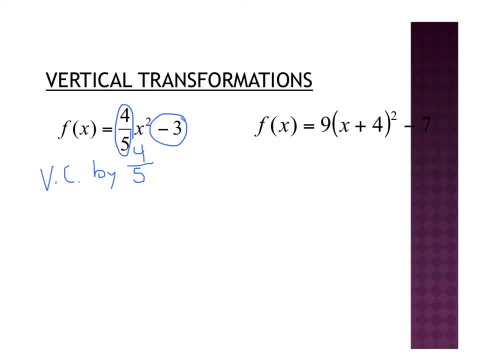 Therefore, it's again a vertical. so up or down. In this case we're going down by 3.. Let's take a look at the next one Here, one thing at a time, remember. so we have that 9 out in front. Well, that is a vertical stretch because it's greater than 1..